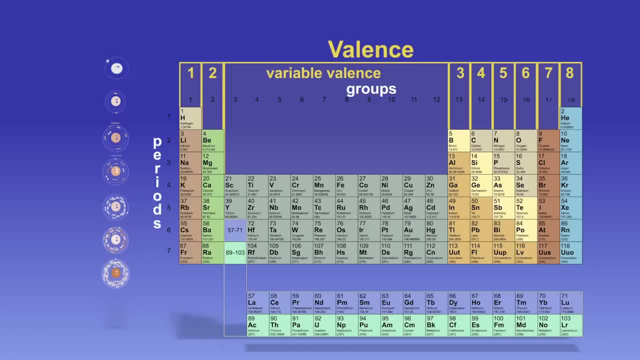 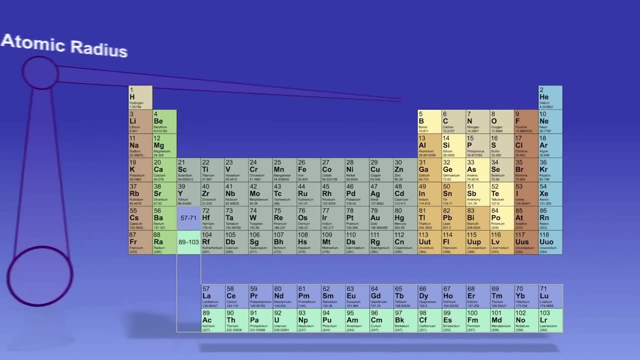 but notice that as you move down through the periods, the number of electron shells will increase. Another trend you will notice is the size of the atom or the atomic radius. As you move down through the periods, the atoms become larger, increasing the atomic radius. 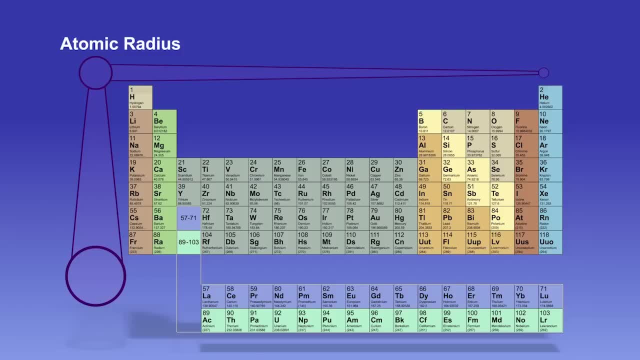 As you move from left to right across the groups, the atoms become smaller, decreasing the atomic radius. The opposite is true for an atom's ionization energy, or how readily an electron can be removed from an atom As you move down through the periods. 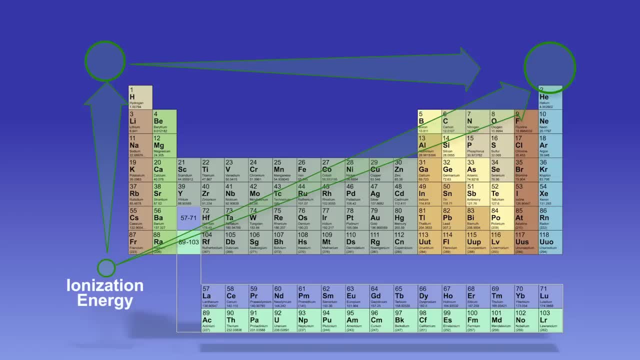 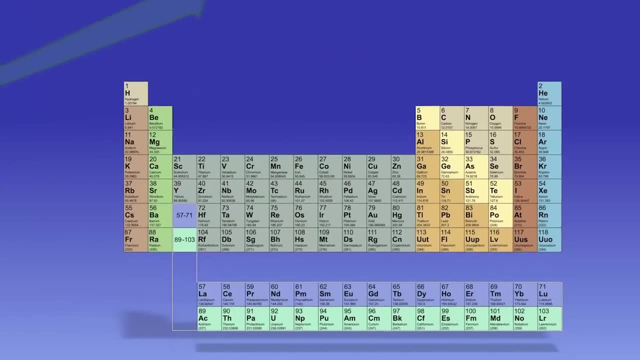 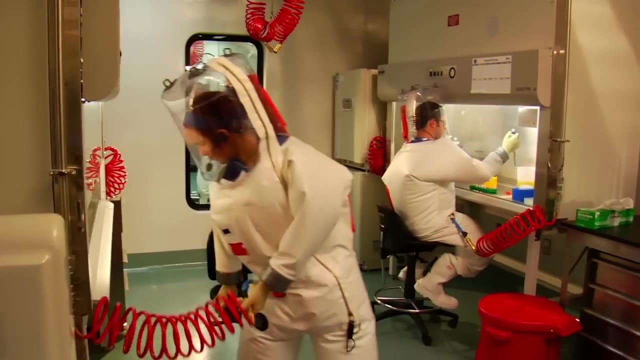 the ionization energy will decrease. As you move from left to right, across the groups, the ionization energy will increase. Knowing the basic properties of the periodic table will be beneficial to you throughout your school career. The periodic table allows scientists to determine the atomic structure of elements. 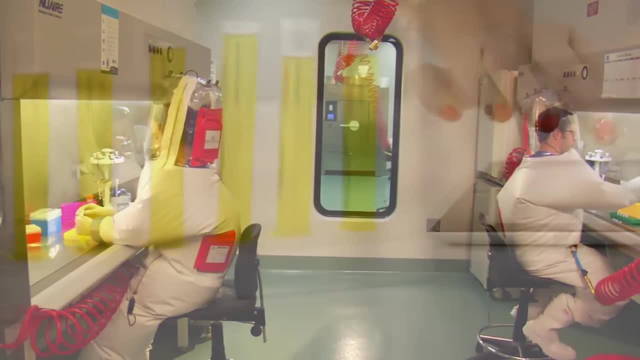 and predict how they might behave. Once you have a firm understanding of the periodic table, you will be able to apply it to experiments in your own classroom. 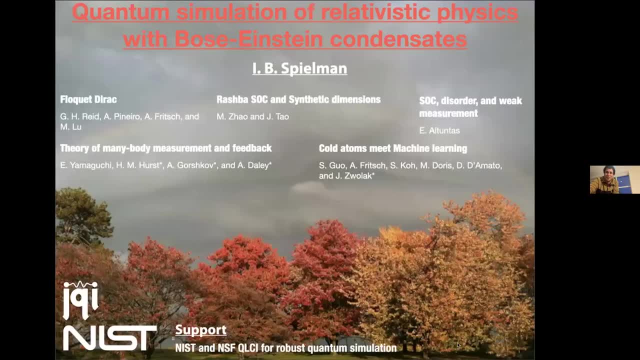 In the center. I have the honor of introducing Ian Spillman, our speaker for today. Before I start doing that, let me also thank Patty Fox, who's been making sure everything is happening just right in the background. I myself am from Caltech and Ian is a graduate of Caltech. He graduated in 2004,.